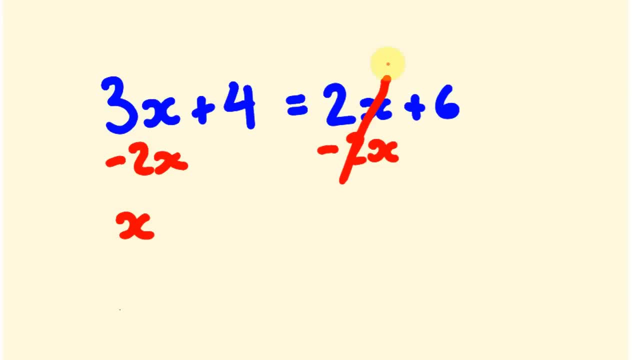 Okay, I also want to get this 4 on this side. So to do this- at the moment it's a positive 4, I'm going to take it off both sides, Okay. so 4 take 4, it's cancelling out, and 6 take away. 4 is 2.. 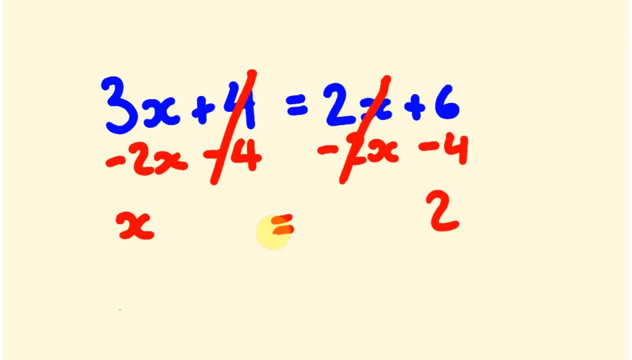 Now that's the way we generally solve these, but you can probably see that we can skip a few steps here. Okay, we don't really need to actually take away 4 off this side as obviously as we do it here. Pretty much all we do here is- I'll look at the often, just look at the sign here- this positive 4.. 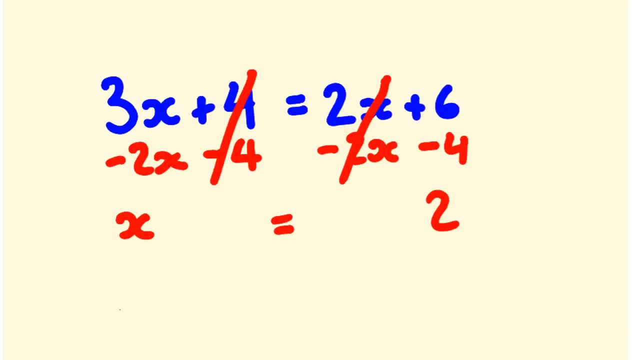 And I take it off the other side and just get rid of it. here I'll show you what I mean. Okay, same question and we'll do it just a little bit faster. and then we'll go through a few other examples. 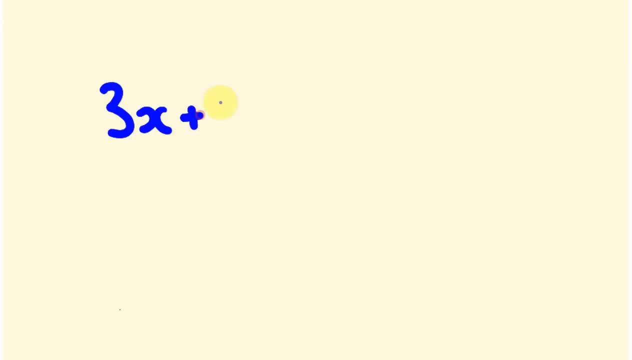 So say we had a. where is it? We have? 3x plus 4 equals 2x plus 6.. Okay, so I want to get the 2x on this side, so it's just a positive 2x. 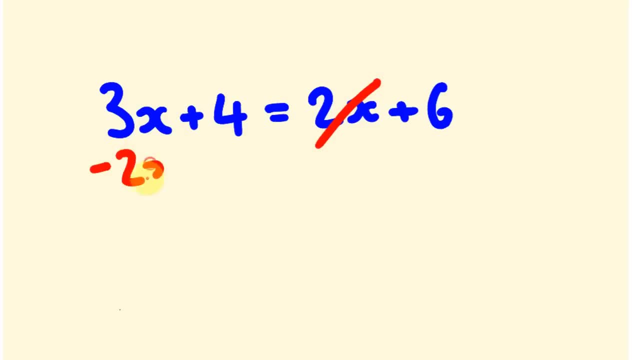 I'm just going to take it off here. okay, because I'm going to cancel it out. If I take it off here, it's going to cancel out straight away. I want to put this 4 over here, so I'm going to get rid of it there and on this side, I'm just going to take it away. 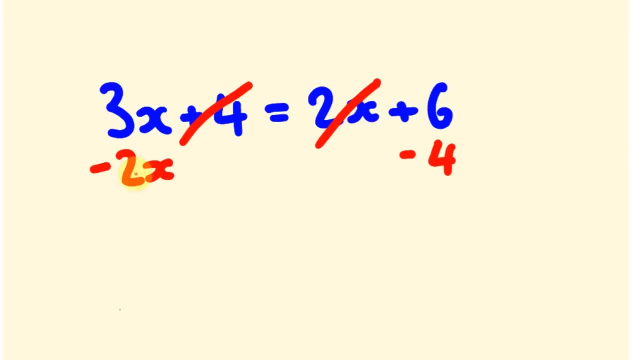 Do the opposite here. So what we're going to end up with is 3x. take away 2x. we end up with x and 6. take away 4, x equals 2.. Okay, pretty easy, right. 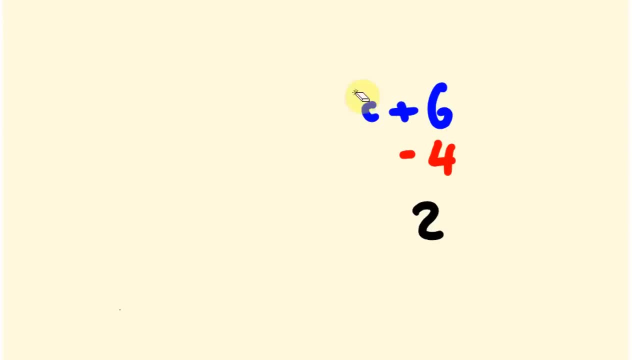 Alright, I'll tell you what we'll go through. another example here: Okay, so say we had 2x plus 1 equals 4x. take away 9.. Okay, so we're going to do that same thing. I like to get all the x's on this side and all the other numbers on this side, so we'll do it like that. 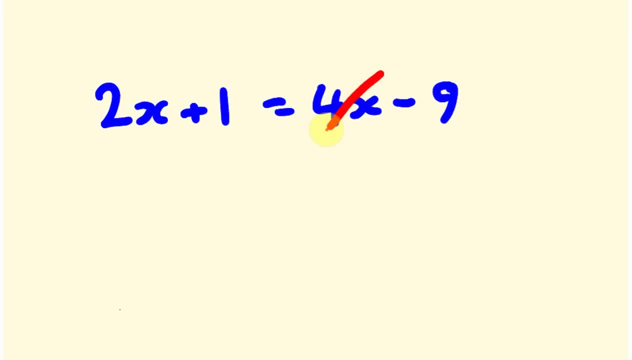 Okay, so I'm going to get rid of this 4x and get it on this side. So to get rid of it, it's a positive at the moment. I'm going to take it away, I'm going to take it off this side. so minus 4x. 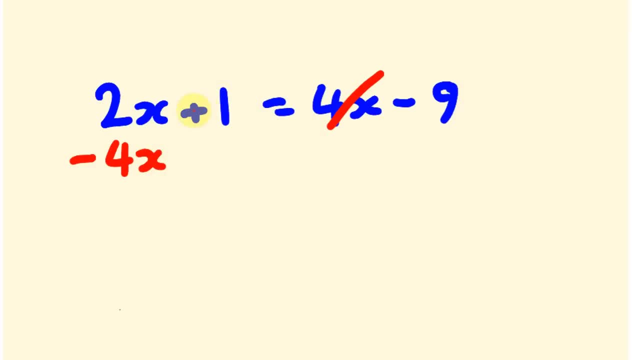 Alright, I want to put this 1 on this side. it's a positive 1 at the moment and I'm going to take it off both sides, so take off 1.. Okay, so 2x take away. 4x is minus 2x. 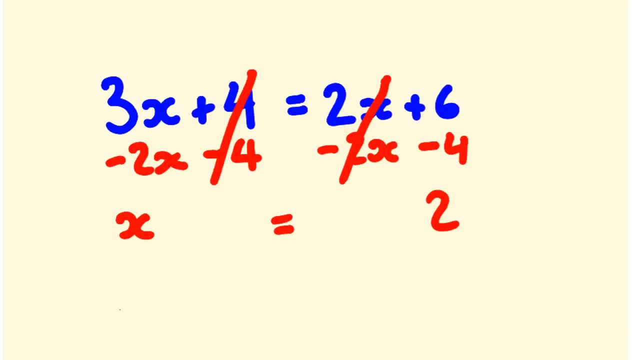 And I take it off the other side and just get rid of it. here I'll show you what I mean. Okay, same question and we'll do it just a little bit faster. and then we'll go through a few other examples. 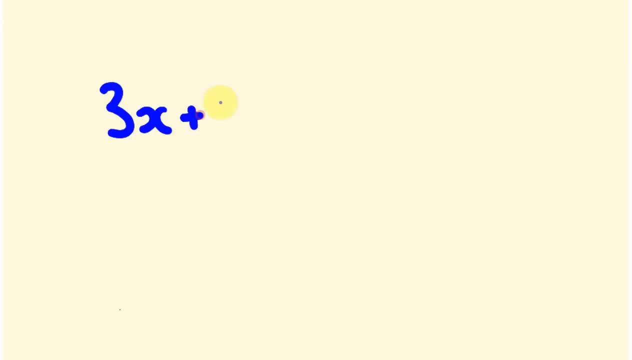 So say we had a. where is it? We have? 3x plus 4 equals 2x plus 6.. Okay, so I want to get the 2x on this side, so it's just a positive 2x. 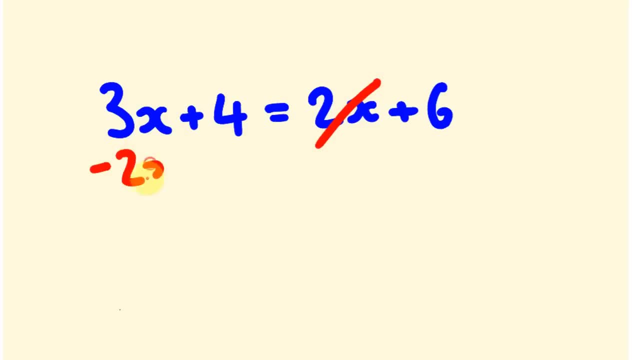 I'm just going to take it off here. okay, because I'm going to cancel it out. If I take it off here, it's going to cancel out straight away. I want to put this 4 over here, so I'm going to get rid of it there and on this side, I'm just going to take it away. 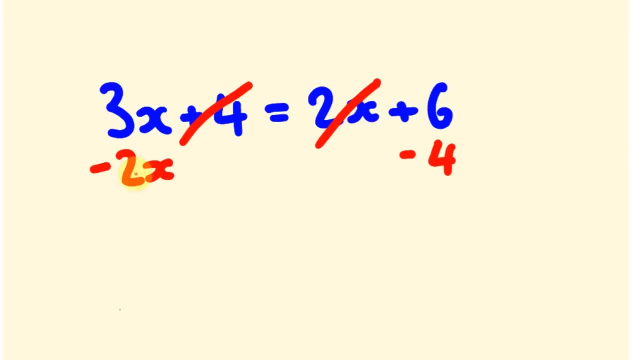 Do the opposite here. So what we're going to end up with is 3x. take away 2x. we end up with x and 6. take away 4, x equals 2.. Okay, pretty easy, right. 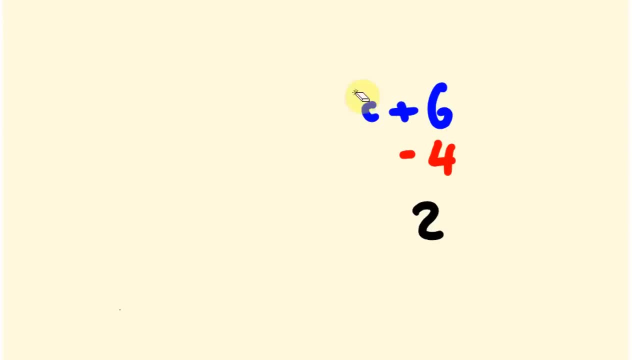 Alright, I'll tell you what we'll go through. another example here: Okay, so say we had 2x plus 1 equals 4x. take away 9.. Okay, so we're going to do that same thing. I like to get all the x's on this side and all the other numbers on this side, so we'll do it like that. 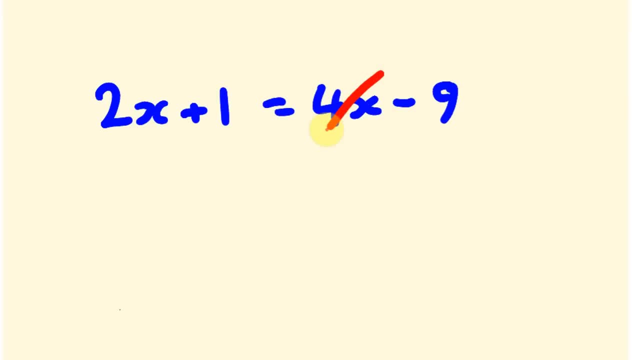 Okay, so I'm going to get rid of this 4x and get it on this side. So to get rid of it, it's a positive at the moment. I'm going to take it away, I'm going to take it off this side. so minus 4x. 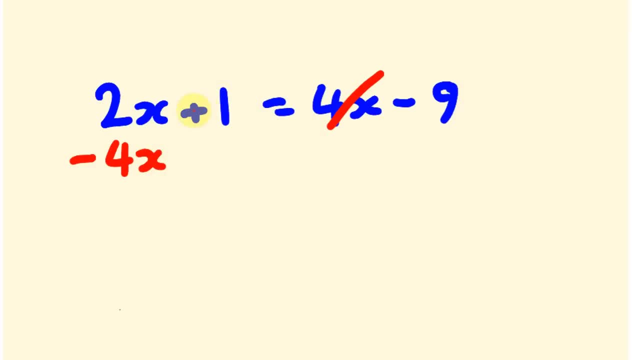 Alright, I want to put this 1 on this side. it's a positive 1 at the moment and I'm going to take it off both sides, so take off 1.. Okay, so 2x take away. 4x is minus 2x. 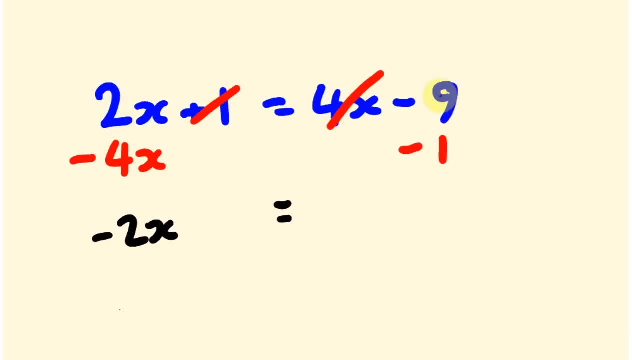 Okay, be very careful with that. Okay, and minus 9 minus 1 is minus 10.. Okay, so pretty much, if we end up with a minus in both of these, we can multiply both sides by minus 1 and get rid of them. 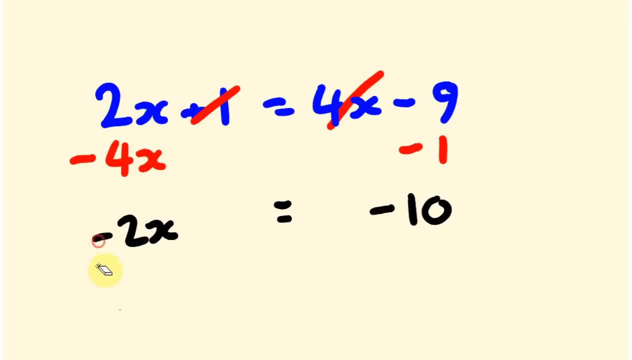 So if we've got a minus on both sides, I can just get rid of this, get rid of that, get rid of that. So 2x equals 10.. This means that x equals 5.. Okay, pretty easy, right.